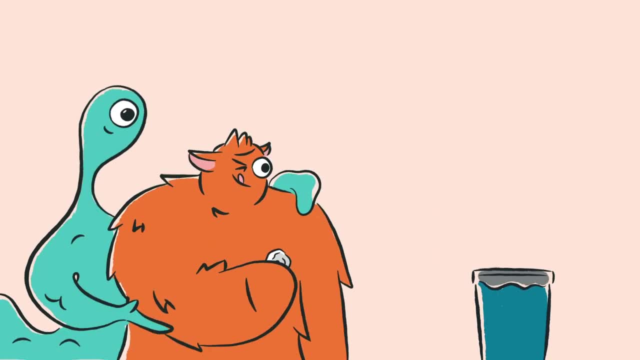 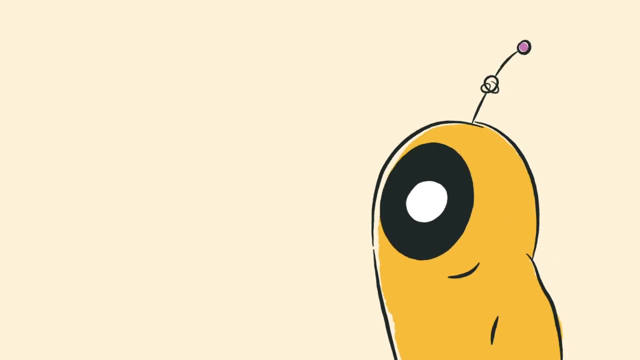 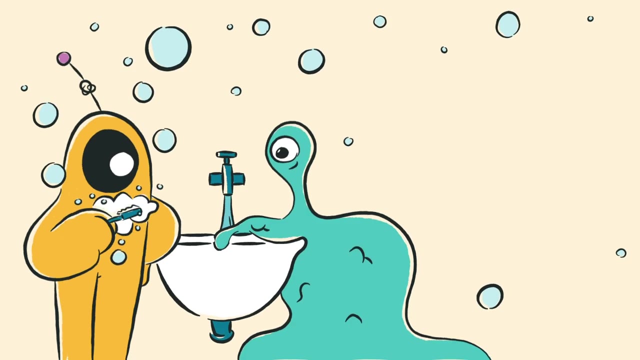 and I can show you why. Pick up rubbish off the ground and toss it in the bin. If everybody does their bit, then all of us can win. Let's be green together. It's easy. if you try, Yellow can be green, said Morph, and I can show you why When you brush your teeth. 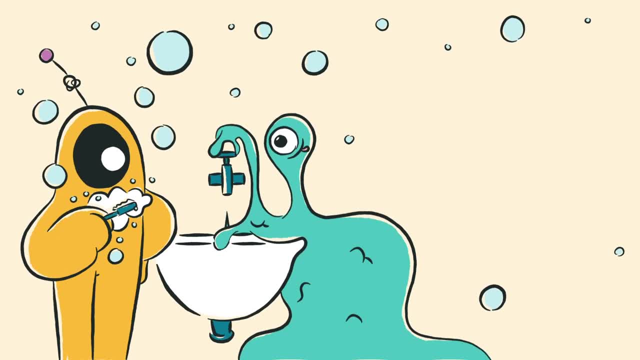 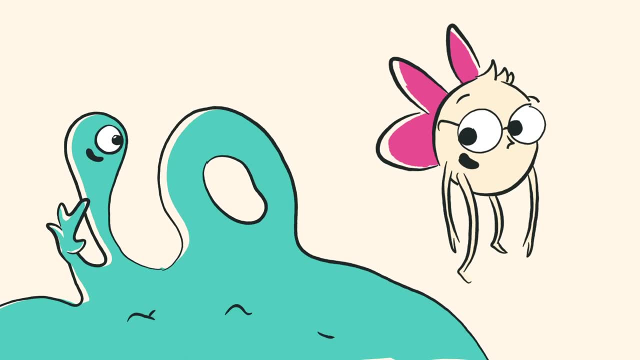 don't leave the tap on. That's a waste. Once the water's down the drain, it cannot be replaced. Let's be green together. It's easy if you try. Coral can be green, said Morph, and I can show you why. 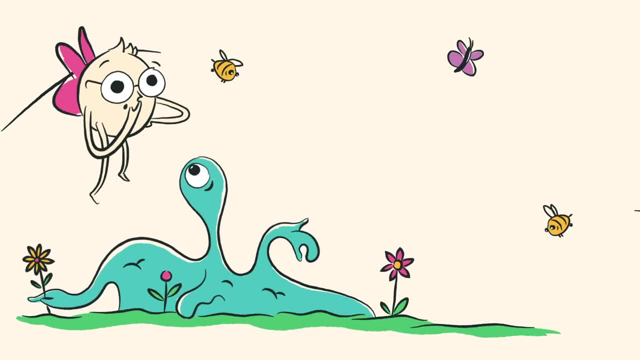 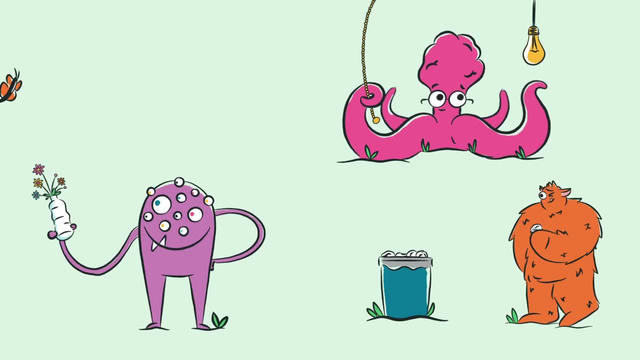 Make some space at home to plant some flowers, herbs or trees. It's fun to do and makes a home for butterflies and bees. We may be small, but each of us together plays a part. These actions make a difference and today's the day we start. All our actions will add up. There's so much we. 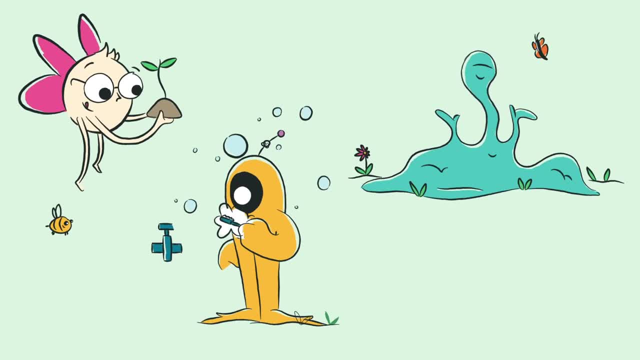 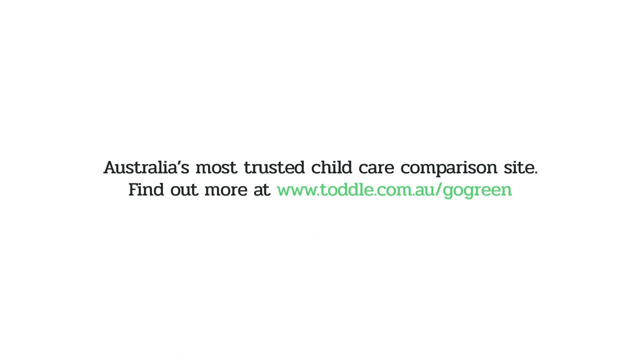 can do. Let's all go green together, and the change can start with you. Let's all go green together. 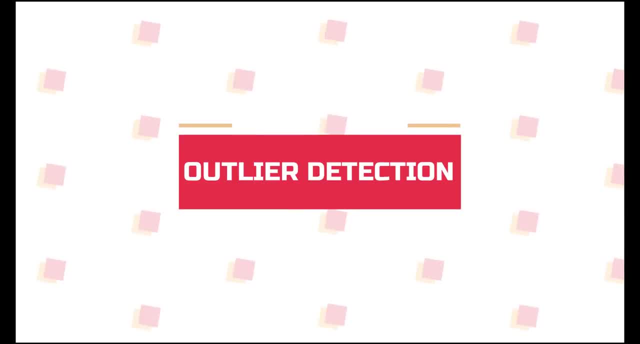 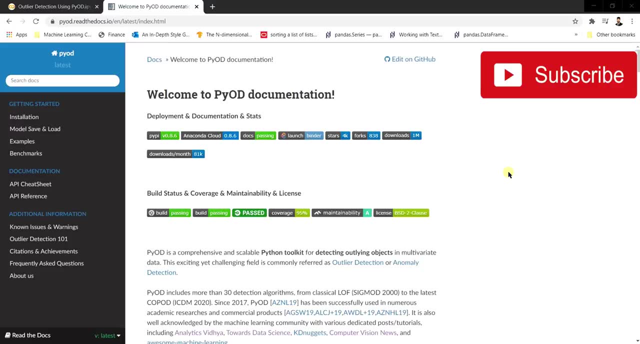 Hello all and welcome to my YouTube channel. So today, in this particular video, I'm going to be talking about an effective way of detecting outliers using PyOD library. So let us start. So, as you can see, the documentation of PyOD has been opened over here, and let us walk. 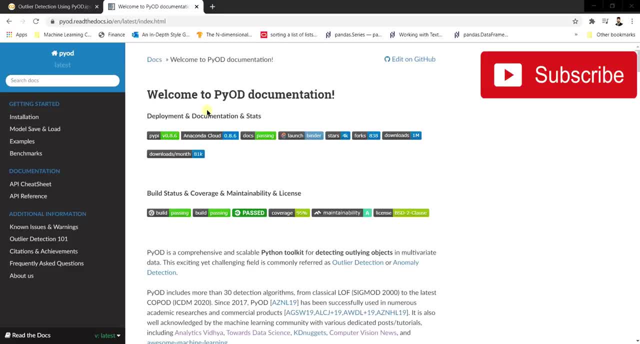 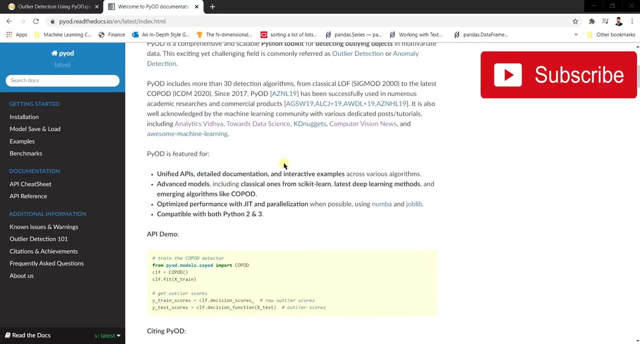 through this documentation before we go through the implementation part of this PyOD. So this PyOD is a comprehensive and scalable Python toolkit for detecting the outliers in multivariate data. So this is an effective library which is generally used in production level for detecting the anomaly as well as outliers. It consists of various kind of algorithms. 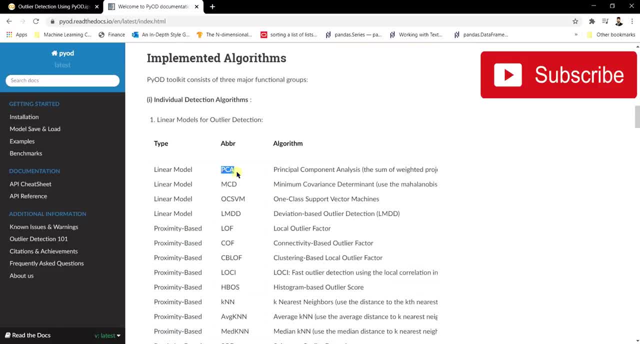 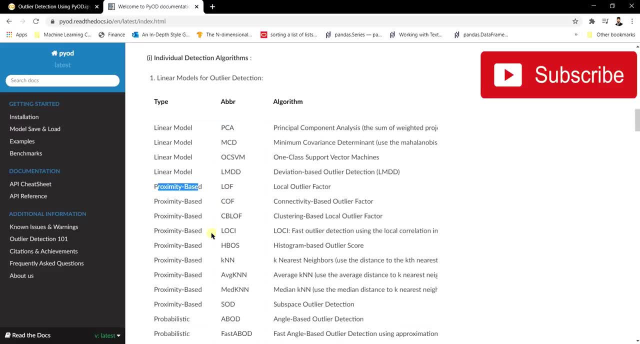 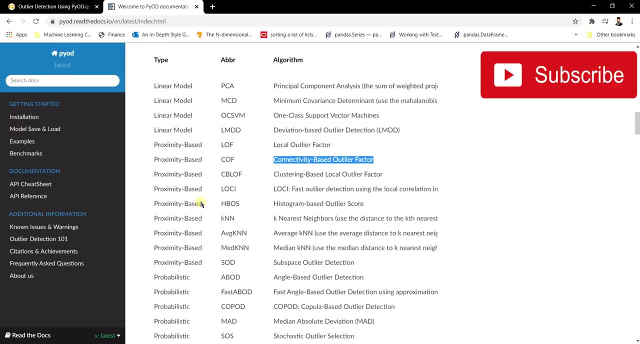 in it. As you can see, it consists of PCA and PCA2.. MCD, which are all are linear models, and there are proximity based models as well, which are such as local outlier factors and connectivity based outlier factors, LOCI, which is fastest.